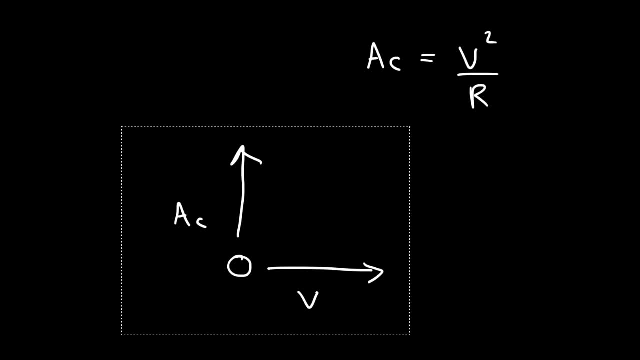 divided by R, where V is the speed and R is the radius of the circle. if you increase the speed of an object while it's moving in a circle, the centripetal acceleration will increase. now, if you double the speed, by what factor will the centripetal acceleration increase? by 2 squared is 4. so if you double the speed, 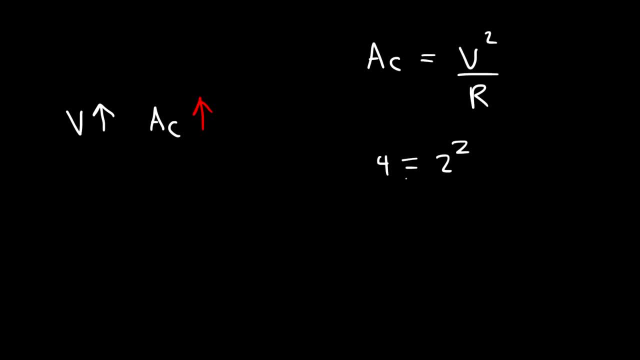 the centripetal acceleration will increase by a factor of 4. if you triple the speed, the acceleration will increase by a factor of 9. now what about the radius of the circle? what's the relationship between a radius and a factor of 9 and the centripetal acceleration? if you increase the radius of the circle, the 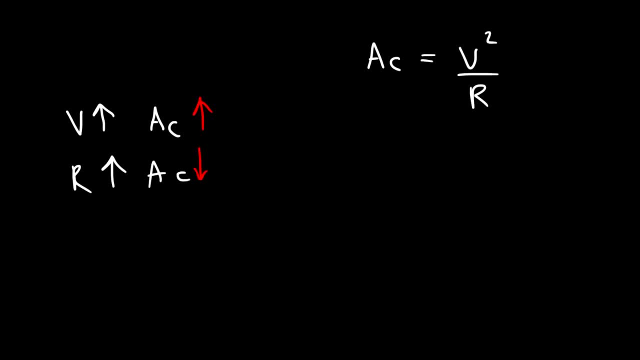 centripetal acceleration will decrease. these two are inversely related. so let's say: if you double the value of R, what happens to the acceleration? to find out anything that doesn't change, plug in 1. if the speed doesn't change, replace it with a 1. since R doubles, plug in a 2. so the acceleration is going to be half of. 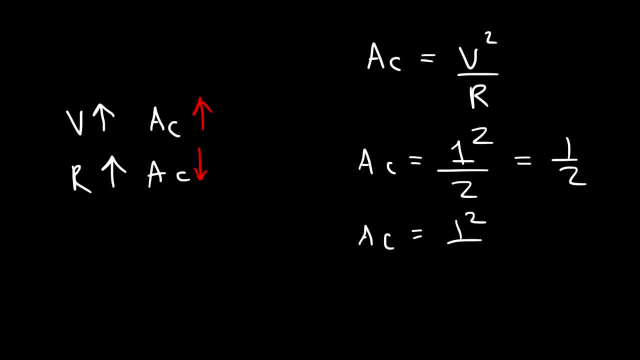 its value. if the radius triples, the acceleration is going to be one-third of its value. now, what if you make the circle smaller? what if you reduce the radius to half of its value? what happens? 1 divided by half is 2. so if you decrease the radius, the 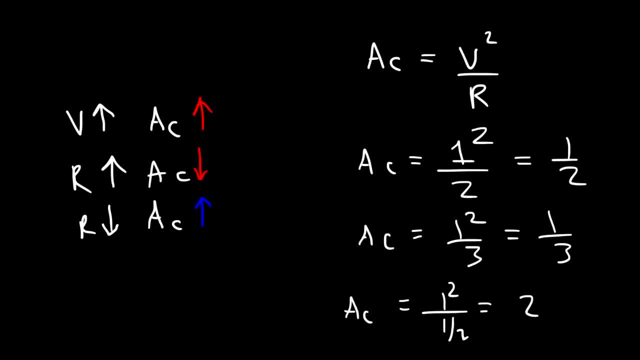 centripetal acceleration will increase. if you cut it in half is going to double. if you decrease it by a factor of 3, the centripetal acceleration will triple. now here's a question for you: what's going to happen if you reduce the radius to one-fourth of its value and 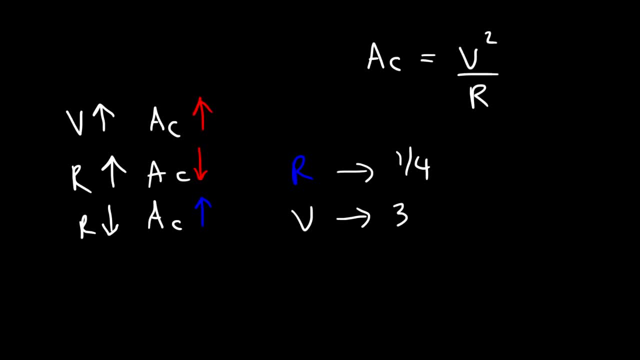 you increase the speed by a factor of 3. what effect will this have on a centripetal acceleration? to find out, just plug it in: 3 squared is 9. 9 divided by one-fourth is the same as 9 times 4. so the centripetal acceleration will increase by a factor of 36. now there's 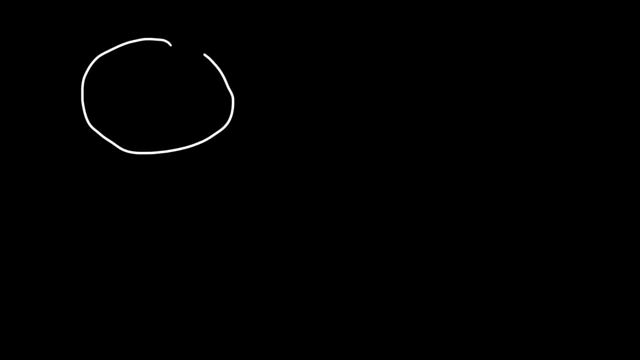 some other stuff you need to know. how do you find the speed of the object if it's moving in a circle at constant speed? by the way, whenever an object moves in a circle at constant speed, the object is moving with uniform circular motion. if the speed is not constant, it's non-uniform circular motion. 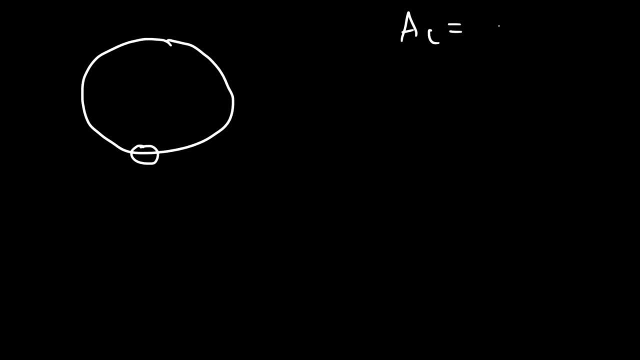 in order to find the centripetal acceleration, you need to be able to determine the speed of the object, because the object is moving at constant speed. there's one equation that we need to know: D is equal to the team, so V is a distance traveled divided by the time. the distance traveled is basically the. distance around a circle equal to time divided by distance traveled. divided by time is basically the distance traveled, is basically the distance around a circle, and the time was disse 40 times� wins place rather than taking advantage of memory dinner. so v is a distance travel two hundred and seven to 50 times. demande is a time rather than aеш ora in signe day. 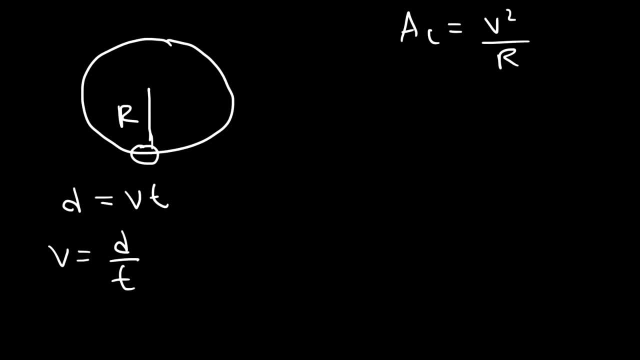 And the distance around a circle is known as the circumference. The circumference of a circle is 2 pi times the radius of the circle And because we're dealing with periodic motion, that's motion that repeats. it goes on forever and ever. you can keep going on around a circle as many times as you want. 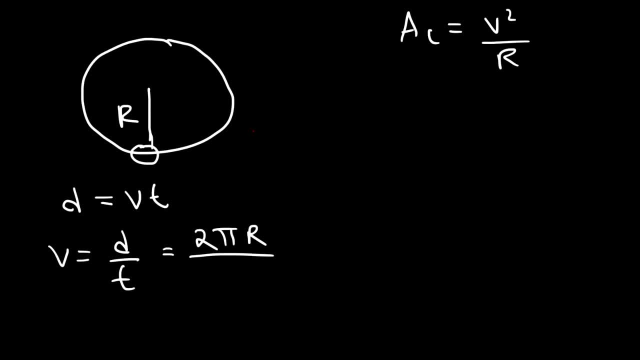 You need to deal with something known as the period. The period is the time it takes to complete one full cycle, And the period is known as capital T. Lowercase t is simply the time it takes to go from point A to point B. 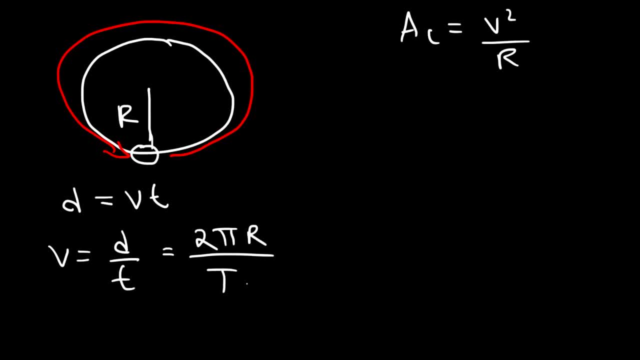 Capital. T is the time it takes to make one revolution, one cycle. So that's the period. Frequency is 1 divided by the period. So let's say, if it takes 0.25 seconds to make one revolution, That would be the period. The period is 0.25 seconds. 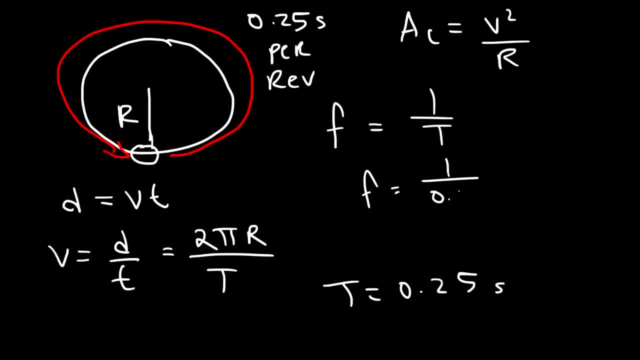 The frequency is 1 over 0.25, which is basically 4.. So if it takes only 0.25 seconds to make one revolution, then you can do 4 revolutions in one second, And that's the frequency. The frequency is the number of cycles that you can complete in one second. 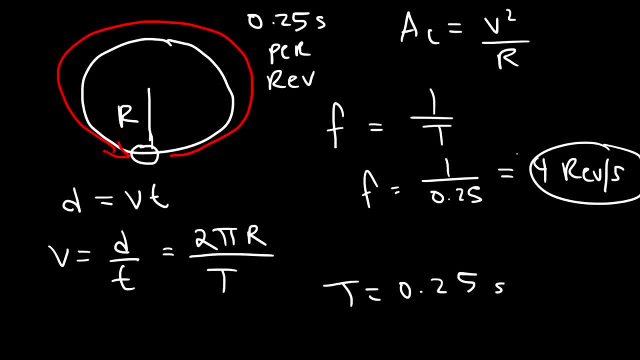 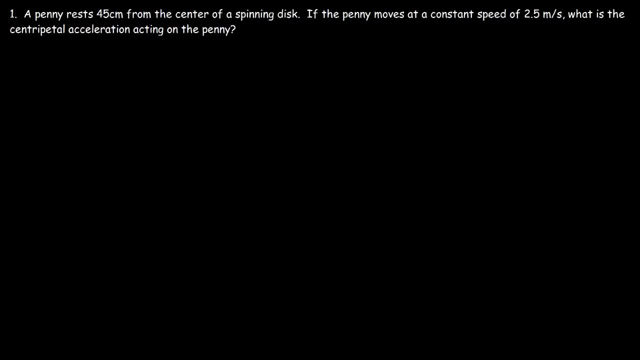 The period is the time it takes to complete just one cycle. Now let's work on some word problems. A penny- A penny rests 45 centimeters from the center of a spinning disk If the penny moves at a constant speed of 2.5 meters per second. 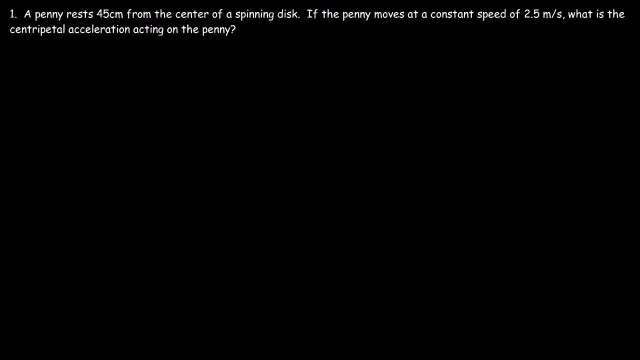 what is the acceleration? the centripetal acceleration, rather acting on the penny. So all we need to do in this problem is use this formula: The centripetal acceleration is the square of the speed divided by the radius of the circle. 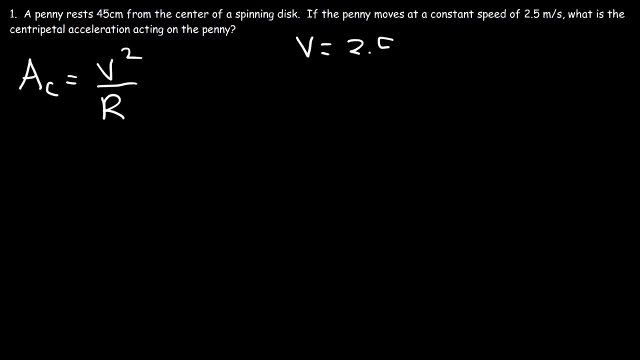 Now we have the speed: V is 2.5.. V is 2.5 meters per second. Now what about the radius of the circle? Now, it rests 45 centimeters from the center of the spinning disk. So that's the radius. 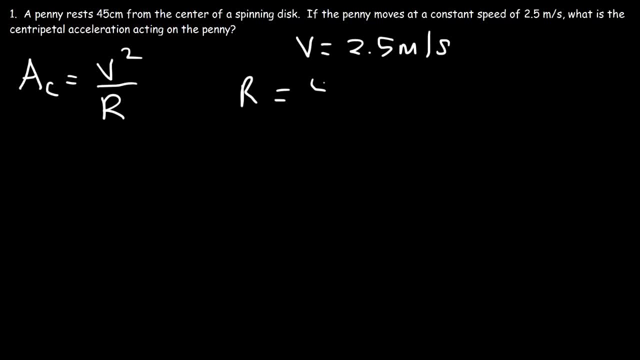 However, we need to convert that to meters. So how can we convert centimeters to meters? It's important to know that 1 meter is equal to 100 centimeters, So all you have to do is divide it by 100.. So 45 centimeters. 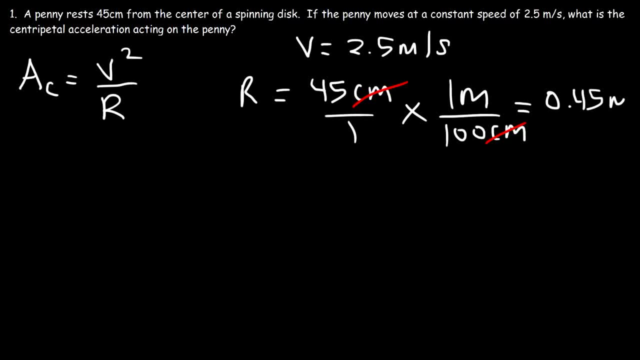 So 45 centimeters is 0.45 meters, So the centripetal acceleration is going to be 2.5 meters per second squared divided by the radius of 0.45 meters, So the acceleration is 13.9, rounded to the nearest tenth, meters per second squared. 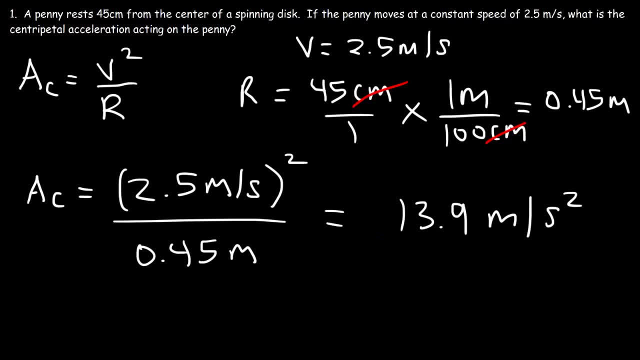 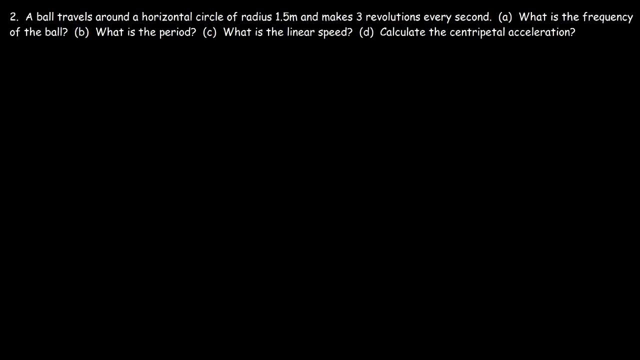 And so that's all you need to do in this problem. Number two, A ball travels around a horizontal circle of radius 1.5 meters and makes three revolutions every second. What is the frequency of the ball? The frequency- Okay, that doesn't look like an F. 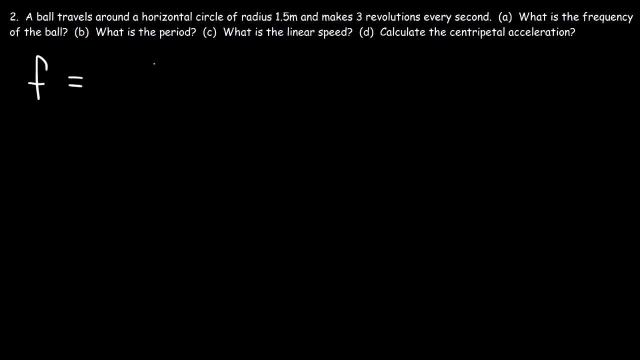 The frequency is the number of cycles Divided by 1.5 meters per second squared, So that's all you need to do in this problem. Divided by the time, So it's the number of cycles that occur in one second. 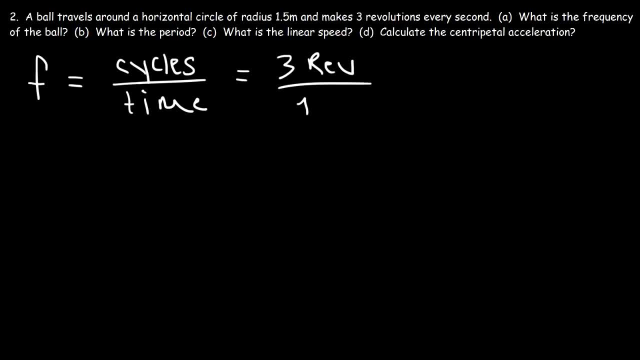 So we have three revolutions, or three cycles. that occurs in one second, So the frequency is just three. It's three revolutions per second. Now what about B? What is the period? The period is the time divided by the number of cycles. So 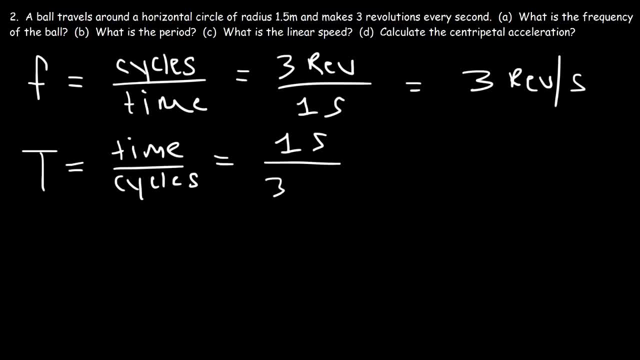 One second. In one second there are three revolutions, Or this ball travels three revolutions in one second, So the period is one over three. You can also find it using this: T is one over F, So if F is three, then T is one third. 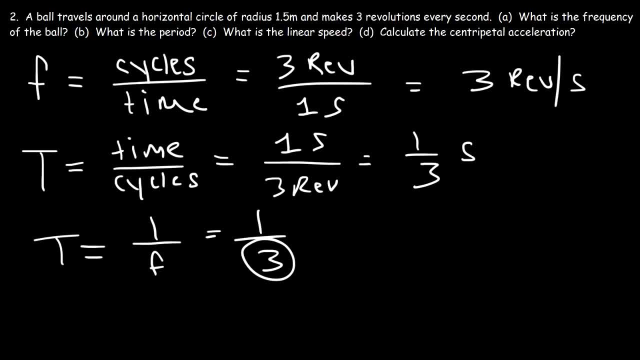 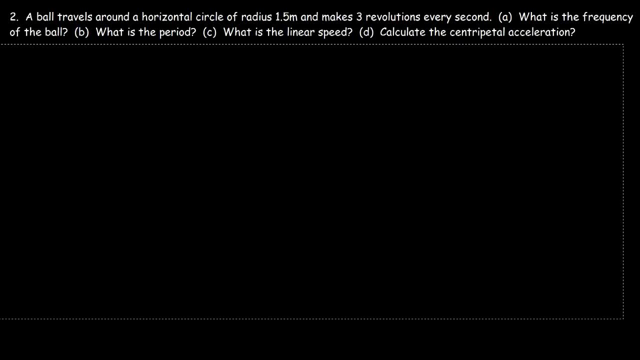 So the period is one third second per revolution. Now, what about part C? What is the linear speed? To find the linear speed, It's going to be two pi R, The distance around the circle Divided by the period, The time it takes to make one revolution around the circle. 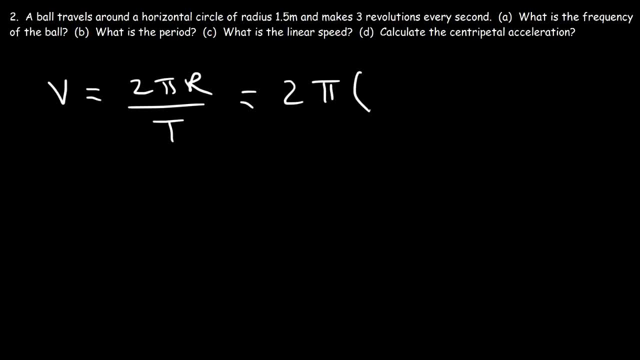 So in this problem we can see that the radius is one point five meters And we know the period is one third of a second. So it's two pi times one point five, Which is three pi Divided by third. So this is equal to nine pi. 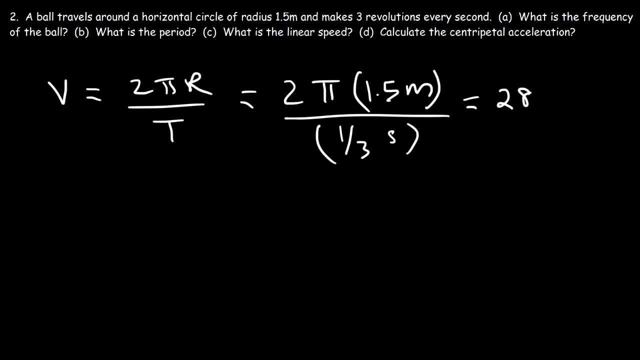 Which, as a decimal, That's twenty eight point two, seven meters per second. So that's the linear speed. So now part D. What is the centripetal acceleration? The acceleration is V squared divided by R, So it's going to be twenty eight point two, seven squared. 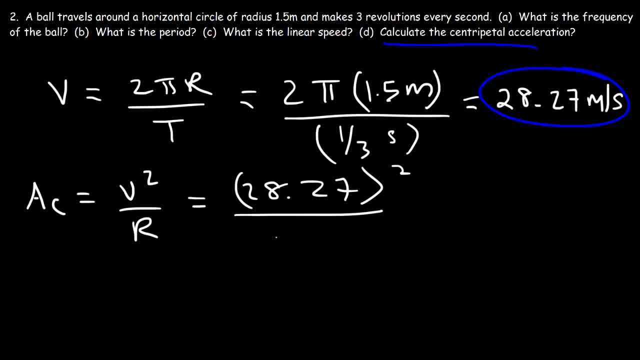 Divided by the radius, Which is one point five, And so rounded to the nearest whole number, It's about five hundred and thirty three meters per second squared. So that's the centripetal acceleration. Now, sometimes You can combine these two equations if you want to. 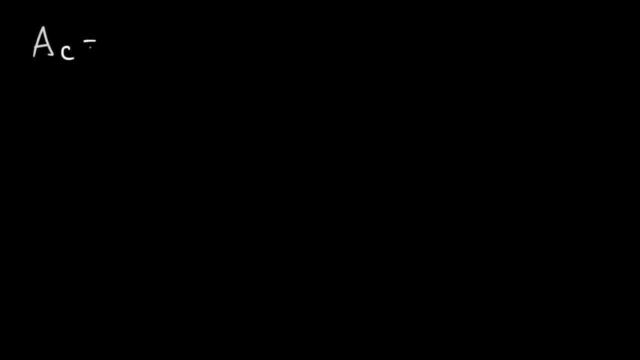 So we have this equation And we know V is two pi R Over T, So I'm going to replace V With two pi R over T, But first I'm going to rewrite it. I'm going to rewrite this as One over R times V squared. 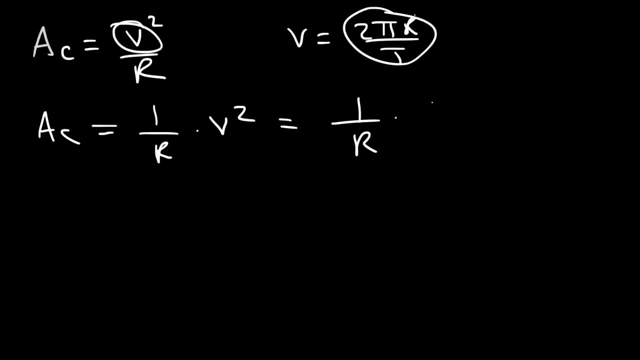 And V squared, That's going to be two pi R Over T squared. Two squared is four. So we got four pi squared Times, R squared Divided by T squared, And so you can cancel an R. So in terms of the radius and the period, 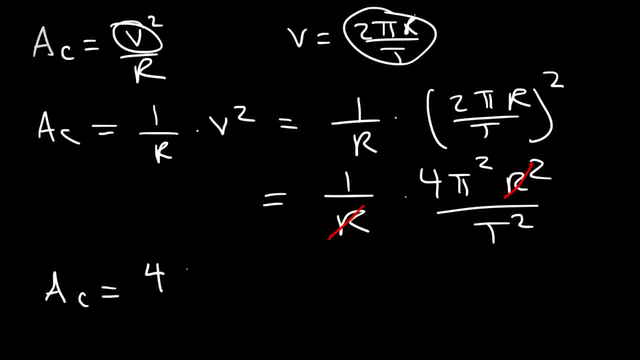 The centripetal acceleration is going to be Four pi squared, R Divided by T squared. So whenever you encounter a problem That gives you the radius of the circle And the time it takes to complete One revolution, You can use this equation. 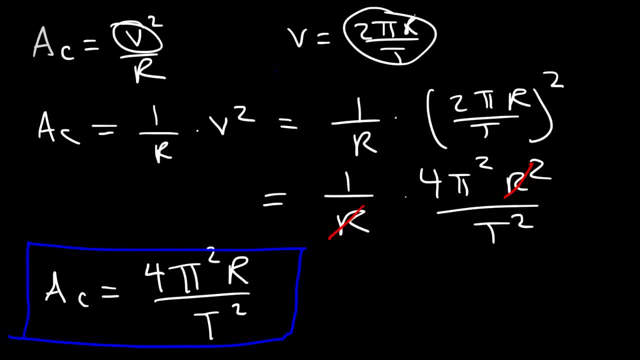 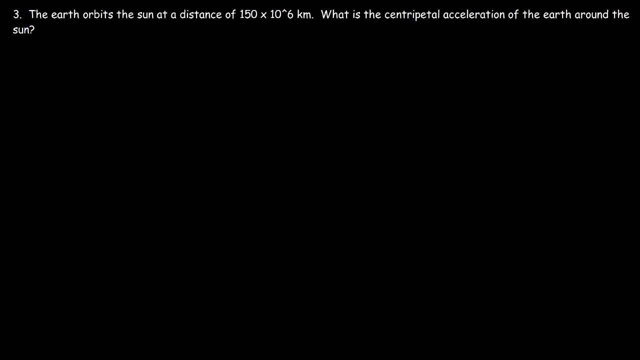 To find the centripetal acceleration directly, Without having to find The linear speed first. Unless you have to find that, Then you can use that. Let's move on to number three. The earth orbits the sun At a distance of 150.. 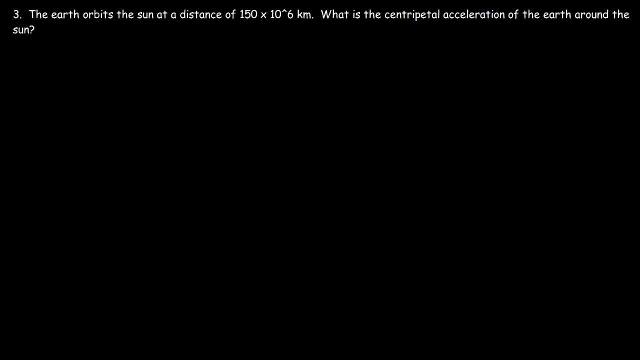 Times 10 to the sixth kilometers. What is the centripetal acceleration Of the earth around the sun? So let's draw a picture, So let's say This is the sun, Let's say that's the earth And we're going to assume that the earth. 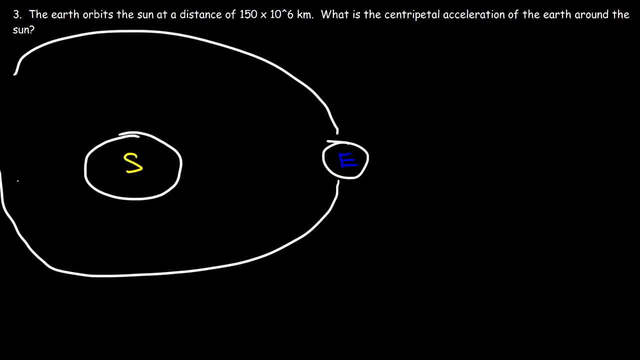 Orbits the sun In a nearly Circular orbit. So what is the centripetal acceleration That's acting on the earth Around the sun? How can we find it? So we have the orbital radius, The distance between Anywhere on this orbit. 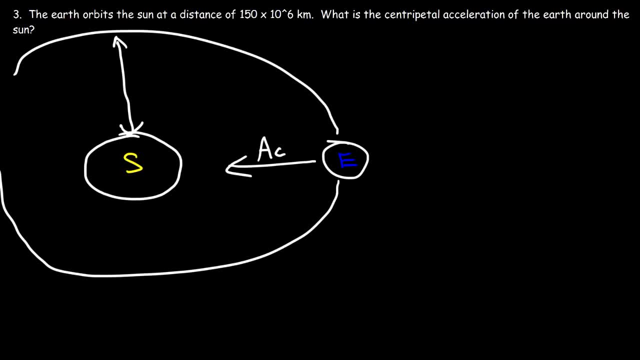 And the earth, And that's equal to 150 times 10 to the sixth kilometers, So that's r. However, we need to convert kilometers to meters And it turns out that One kilometer Is a thousand meters, So 150.. 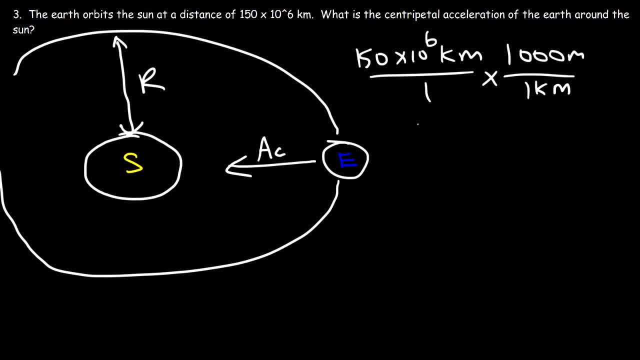 Times 10 to the sixth Times a thousand Is 1.5.. 10 to 11 meters. So that's the radius. Now What other information do we need In order to find the centripetal acceleration? Now recall the last. 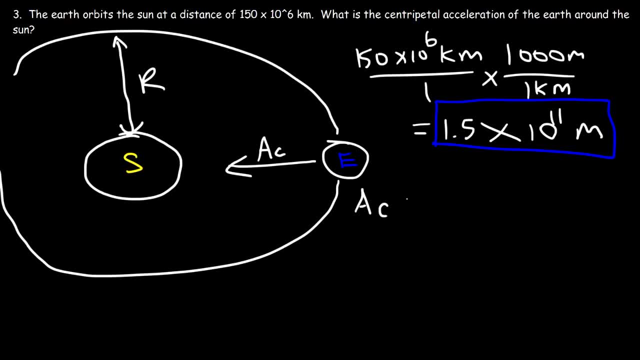 Equation that we used, That we came up with earlier. We said the centripetal acceleration Is 4 pi squared times r Divided by t squared. So we have r And we don't have the linear speed of the earth. 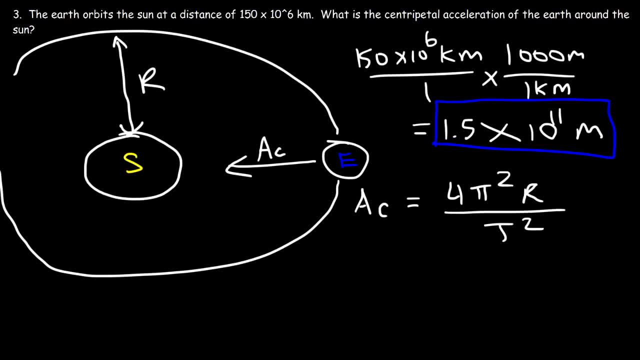 But do we know the period? How long does it take the earth To orbit the sun? It takes the earth One year to make a full trip Around the sun. So the period of the earth is one year, But we need that in seconds. 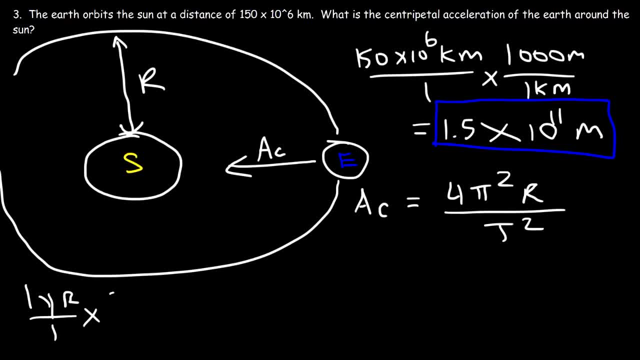 So let's convert one year into seconds. Now we know that There's 365 days In a single year, So the unit years, So the unit years Cancel, And in one day There's 24 hours And within a single hour. 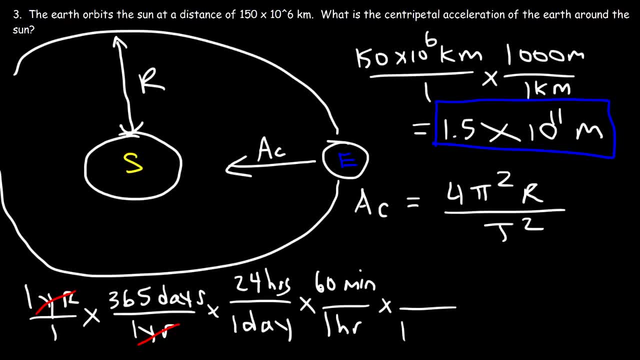 There are 60 minutes And each minute Is equivalent To 60 seconds, So it's 365.. Times 24. Times 60. So the period of the earth In seconds Around the sun Is 31,536,000.. 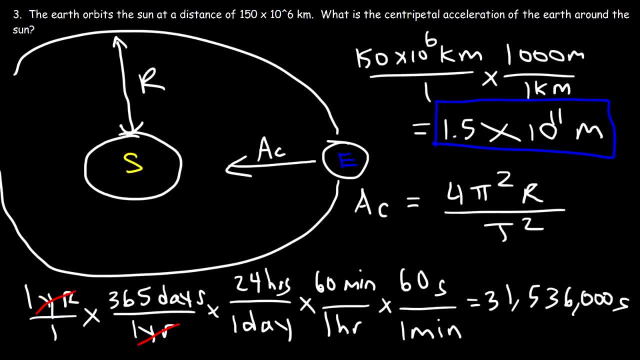 Seconds. So now We have everything that we need To get the answer. Now Let's plug in everything. So it's going to be 4 pi squared Times the radius, Which is 1.5.. Times 10 to the 11.. 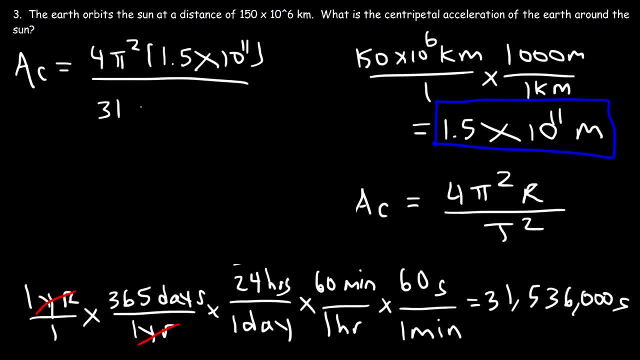 Divided by the period, Which is This big number, But don't forget to square it So. So the centripetal acceleration Of the earth around the sun Is 5.95.. Times 10 to the minus 3.. 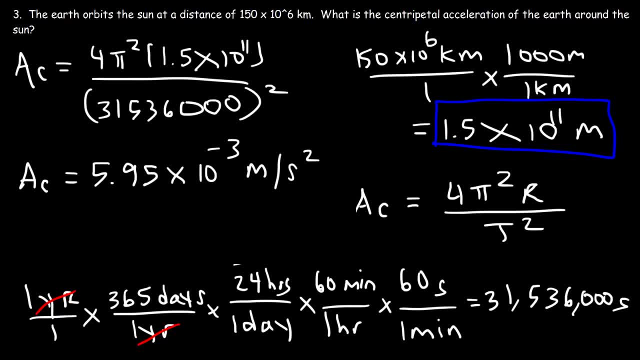 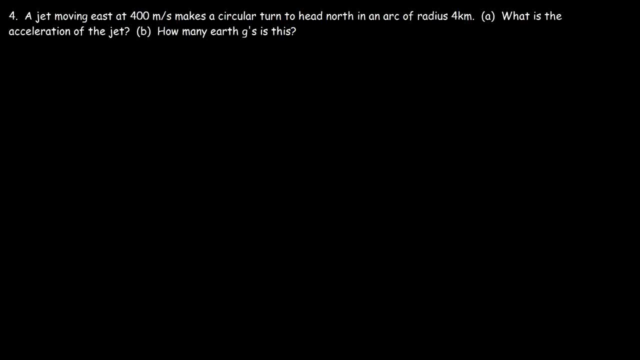 Meters Per second squared. So that's the answer. Now let's move on to our last problem, Number 4.. A jet moving east At 400 meters per second Makes a circular turn to head north In an arc of radius of 4 kilometers. 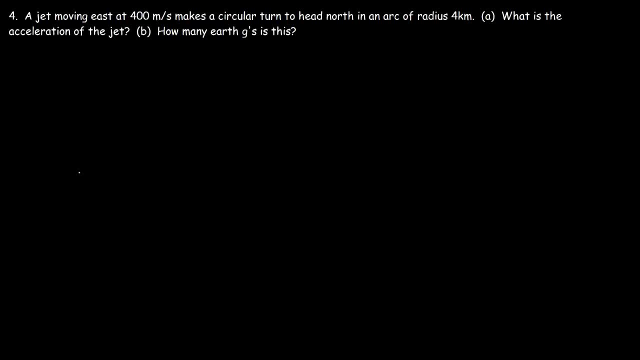 What is the acceleration of the jet? So let's draw a picture. So let's say: This is the jet And it's moving east, And then eventually It's going to make a circular turn To head north. Now the turn is probably going to have to be: 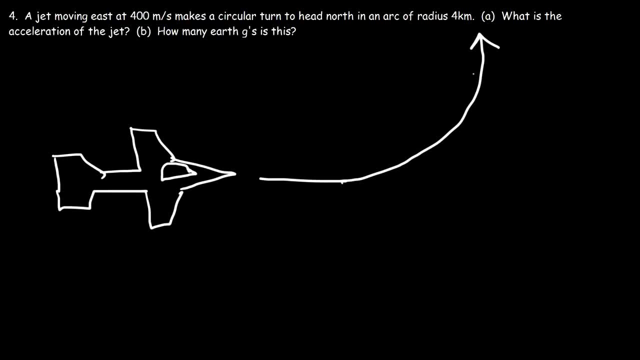 A much wider turn. So right now This is a portion of a circle. Notice that you can Extend the circle if you want to, So that arc Has a circular radius And that radius Is 4 kilometers, So the fact that it's turning. 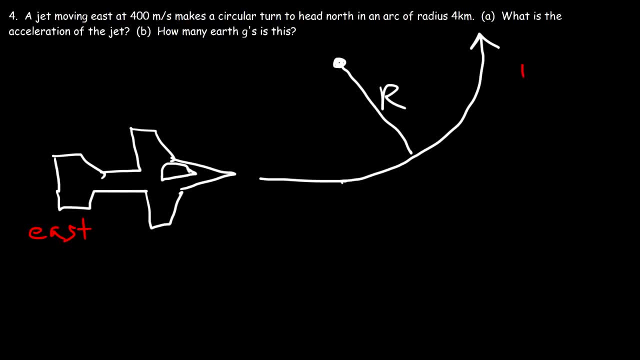 From east to north Means that It's going to experience a centripetal acceleration During that turn. Our goal is to find the acceleration At that point, And we have what we need. We have the velocity, Or rather the speed. 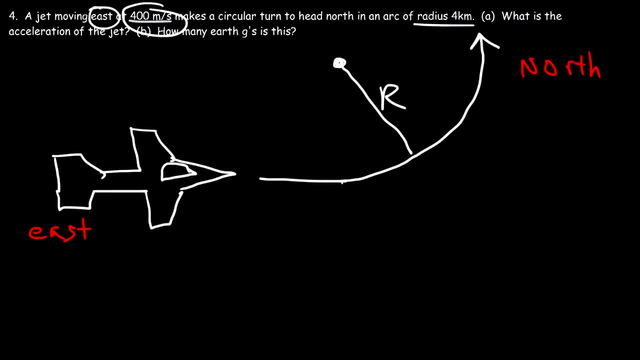 And we have the radius. When you combine the speed with the direction, Then that becomes the velocity. So all we need to do is just use the formula. AC is equal to V squared over R, So V is 400.. And R we need to convert. 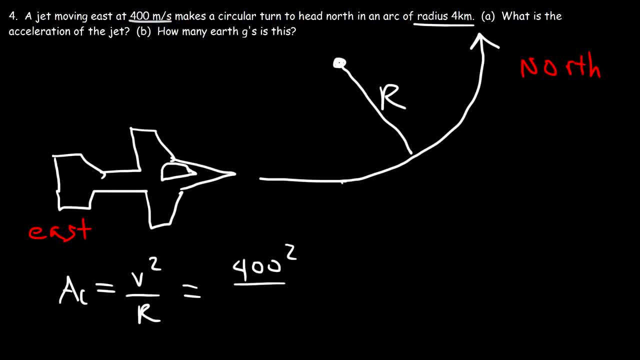 Kilometers to meters. Now, if 1 kilometer is 1000 meters, 4 kilometers Is 4000 meters. So we have 400. Times another 400. Divided by 4000. Where 4000. Is 400 times 10.. 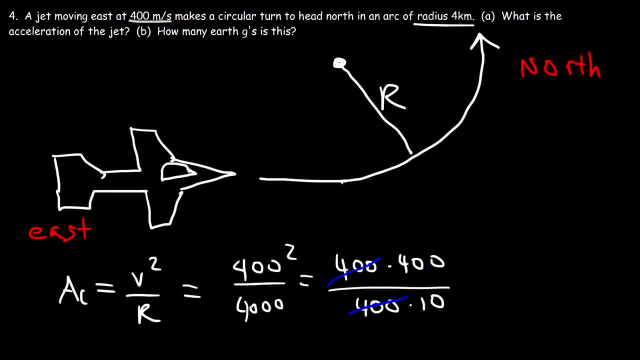 So we can cancel a 400.. And we can cancel, So it's 0.. So it's 40 over 1, which is 40. So the centripetal acceleration Is 40.. Meters per second squared. So that's the answer to part A.